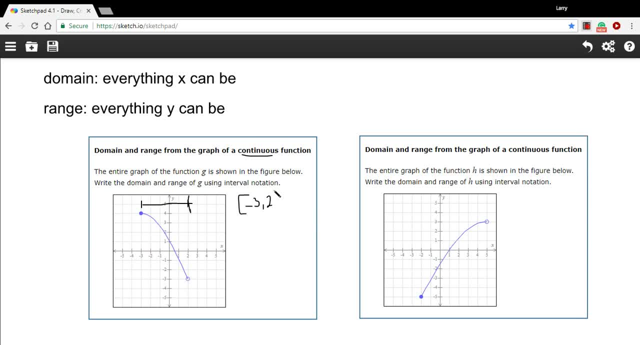 bracket. When you're not including the number in this empty circle, you use the rounded bracket, the parentheses. So this is the interval that describes the domain. So that's domain. Let's figure out range next. So range is the y values which go from up here for all the way down. 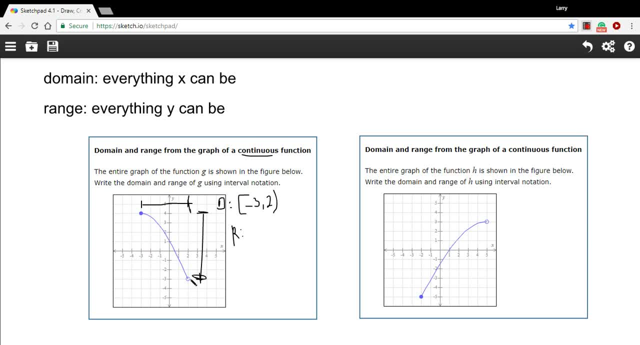 to here, but not including that point there on the bottom. And again we start with the lowest number. So we'll start with negative three And then put a comma, and it goes all the way up to four. The negative three is not included, So we're going to put in a comma And then we're going to put in a comma. 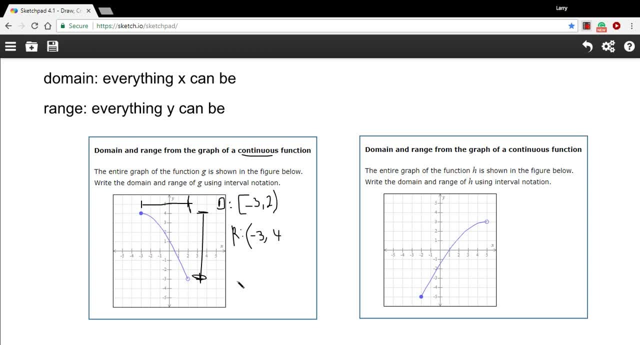 The negative three is not included because that's an empty circle, So we use the rounded bracket. And the four is included because that's a filled circle, So we use the square bracket. So that's the domain and the range in interval notation for this continuous function. 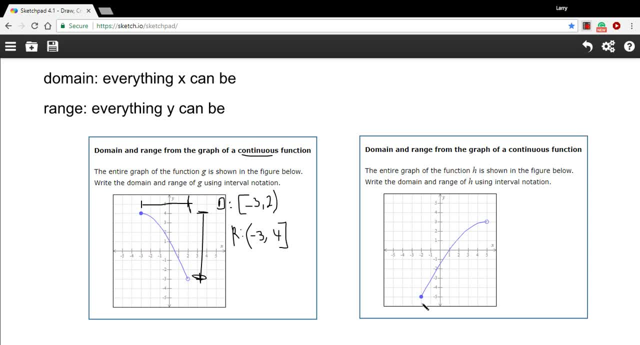 Let's try one more, just for practice. So let's start with the x's. So we begin here, And this is at an x value of negative two, And we go all the way over to here, And that's an x value, So domain from negative two to five, And the negative two is included because that's a filled circle. 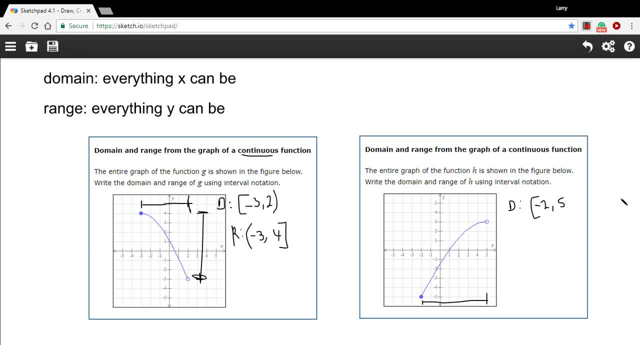 So we use the square bracket. The five is not included because it's an empty circle. So we use the rounded bracket. All right range. So that's the y values, the up and the down. So we can start here at negative five And we go up to, but not including the three. 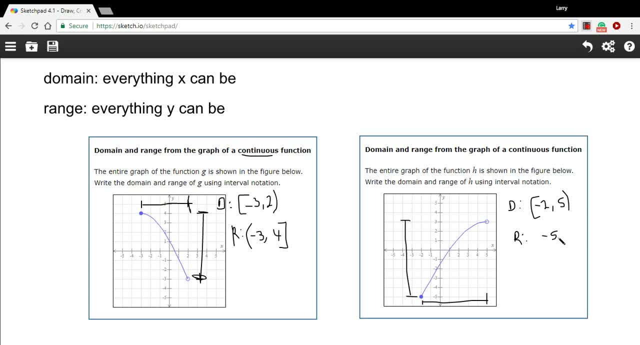 So we just put in a negative five, a comma and a three. The negative five is included, so square bracket, and the three is not, so rounded bracket. So that's how to express the domain and range of a continuous function with interval notation.